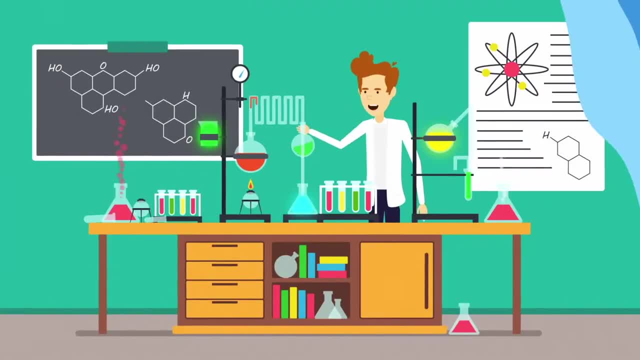 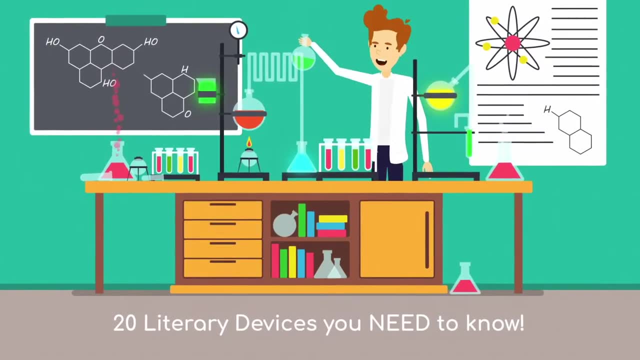 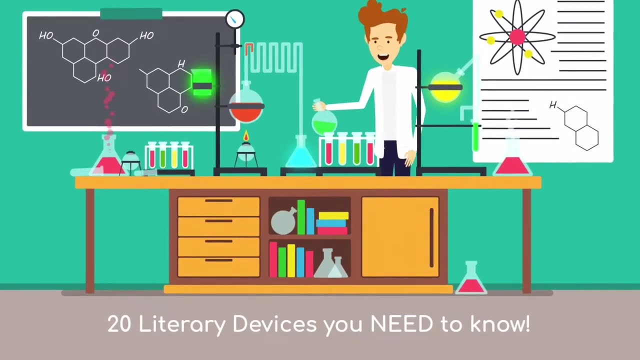 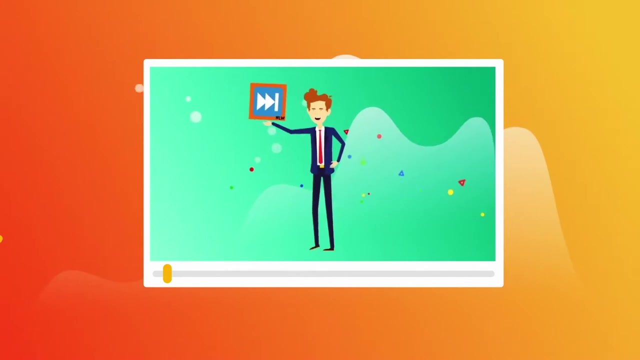 and become a literary device master. Welcome authors to Next Level Writing. This video of 20 literary devices aims to increase your knowledge of literary devices in order to improve your writing and your capacity to review literature. If you find this video helpful, remember to hit the like button and subscribe to the channel. And if you think, one literary device. 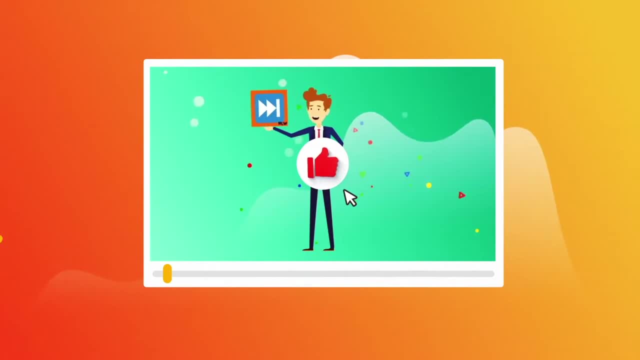 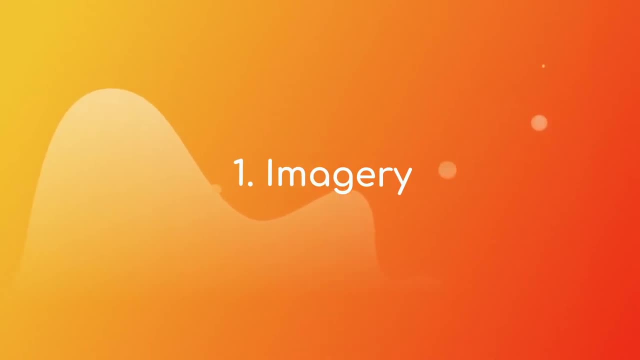 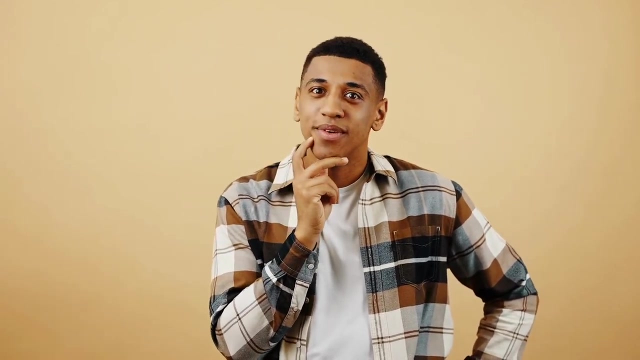 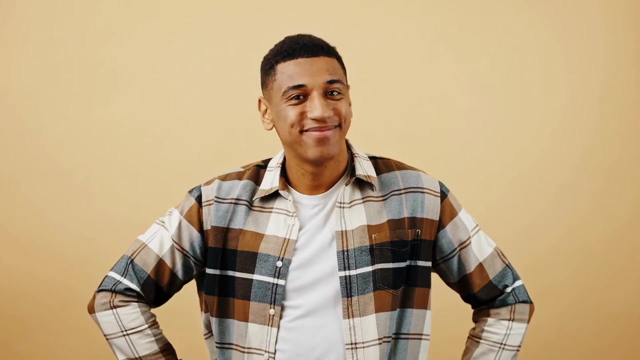 is missing, let us know in the comments section. Without further ado, let's begin our exploration into 20 literary devices. Number one: Imagery. Imagery is a literary device where figurative language is used with the intent to create a picture in the reader's mind. When used effectively, writers can create images by evoking responses. 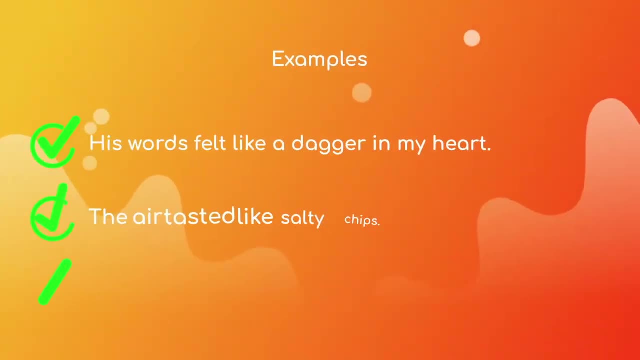 from all of the reader's senses. And here are three examples of imagery. Notice how each of the examples focuses on a different sense in the reader, helping to create a picture in the reader's mind. Number two: Imagery. Number two: Simile. 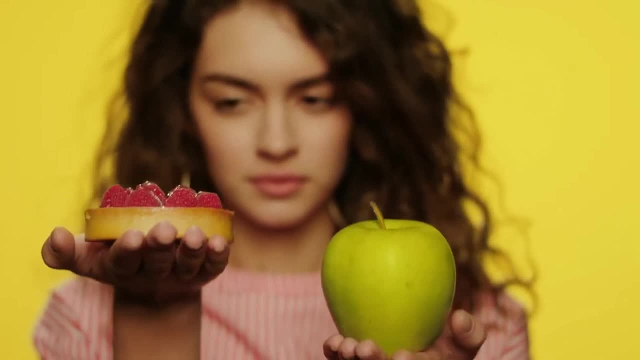 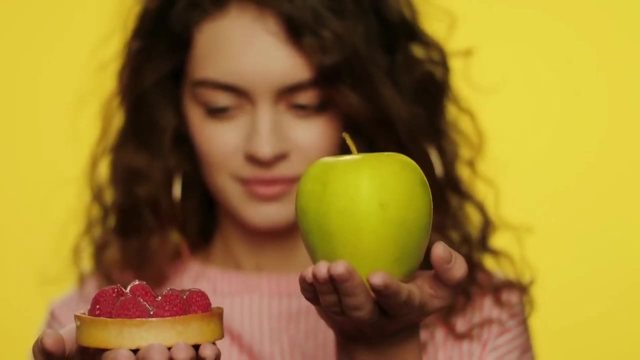 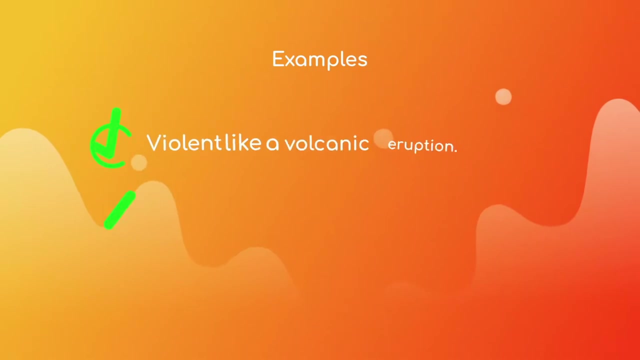 Similes are a figure of speech in which two objects or concepts are compared with one another through the use of like or as. To use a simile effectively, the two things being compared are to be different enough so that the reader will be intrigued by the comparison. And here are three. 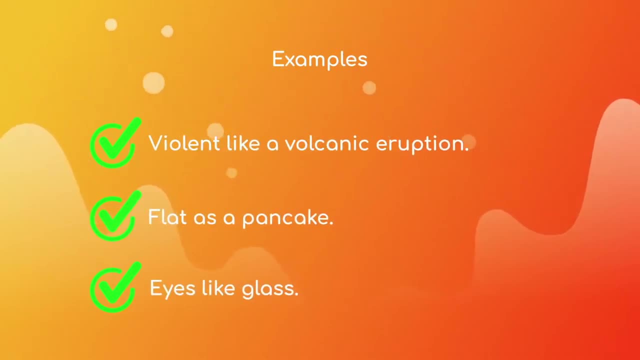 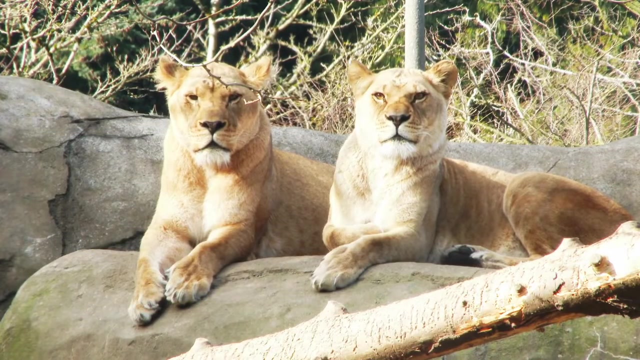 examples of similes. Notice how each of the examples uses the word like or as to compare the two things that are being mentioned. Great similes, indeed. Number three: Metaphor. Metaphors are another figure of speech that makes a comparison between two non-similar things. 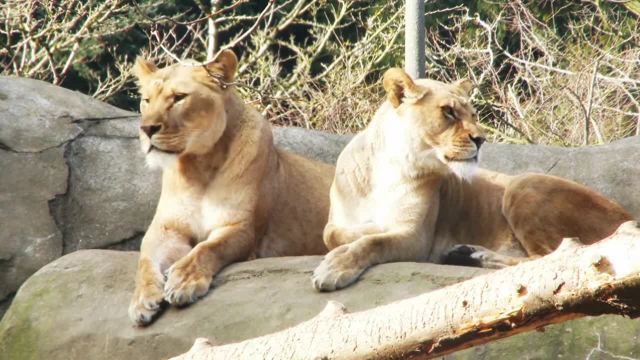 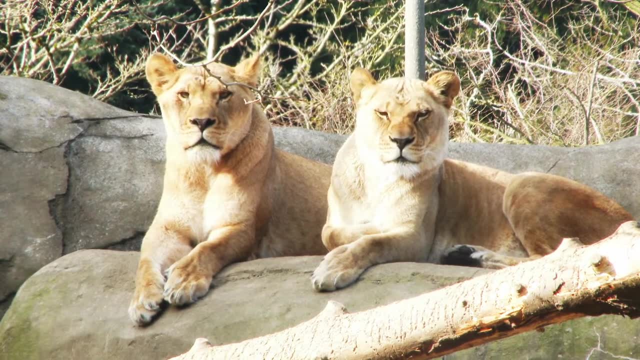 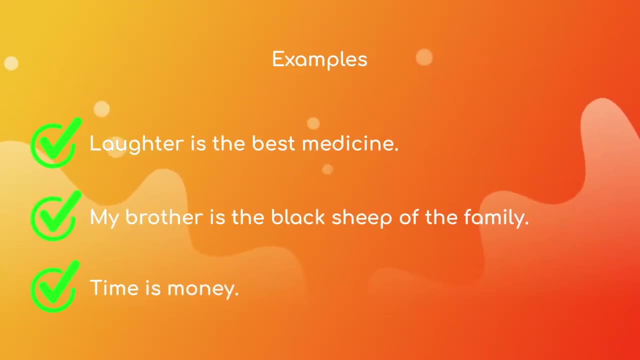 However, unlike similes, metaphors create implicit comparison by not using like or as. By not using like or as, metaphors assert that two things are identical in comparison. rather, And here are three examples of metaphors, Notice how like or as is not used in any. 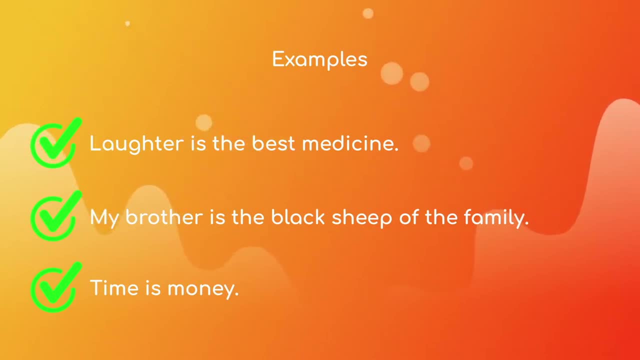 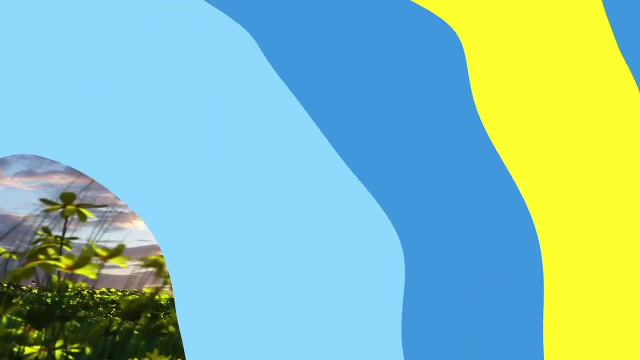 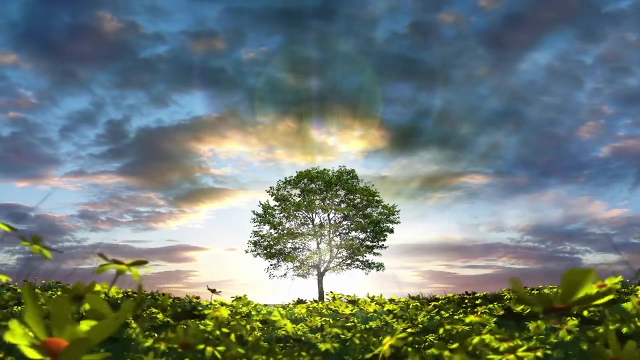 of these examples, meaning that these are great metaphors, by comparing two things. Number four: Personification. Personification is a literary device in which an idea or thing is given human qualities. When using this device, writers make in-depth comparisons between the two things. For example, if a person is